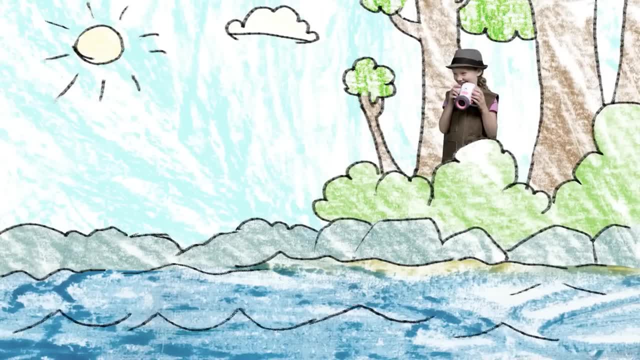 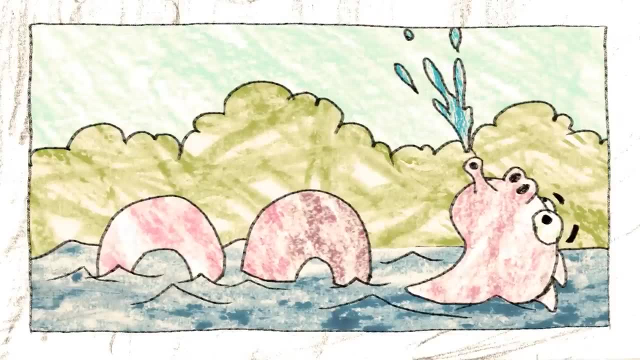 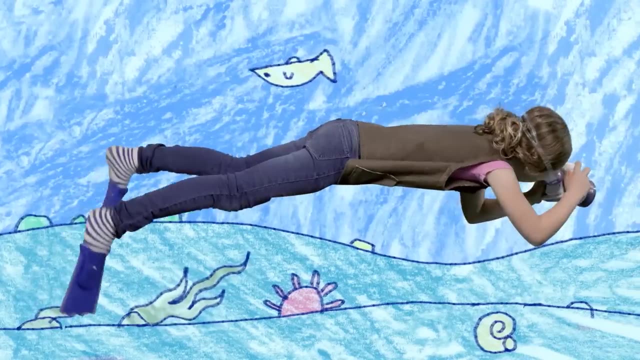 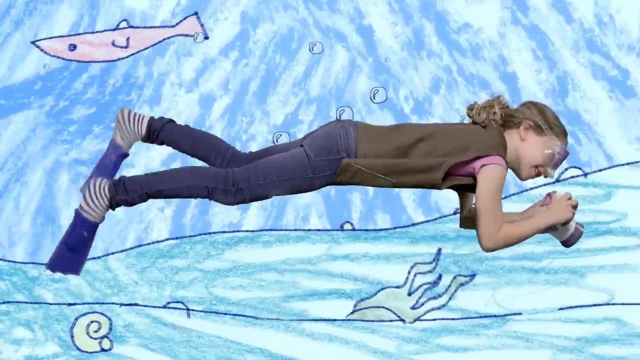 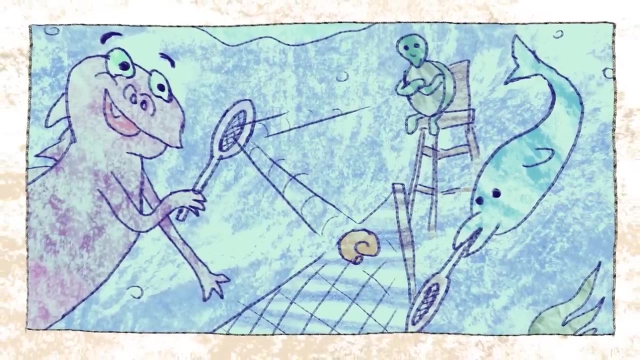 And a sea monster. Sea monsters are pretty cool So I would take lots of pictures to show the whole world. Sometimes I would take underwater pictures for nature websites. The website would want me to take photos of all the different life underwater Selfie. 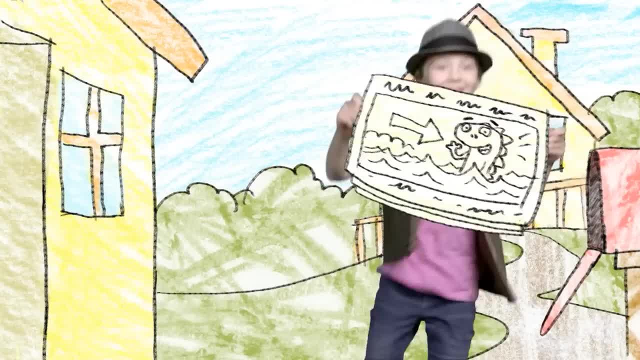 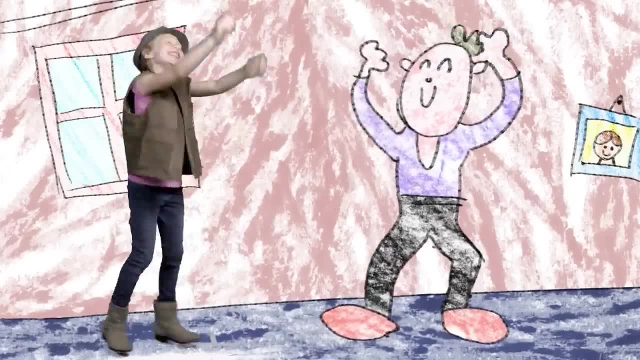 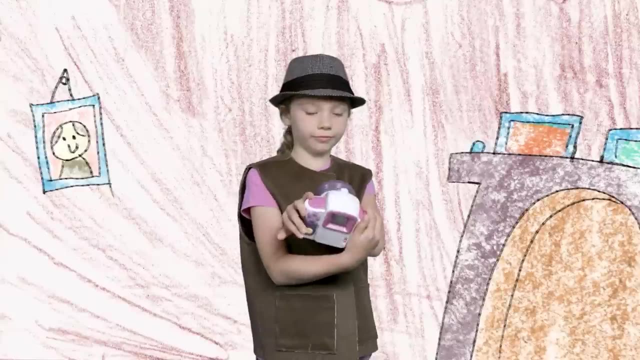 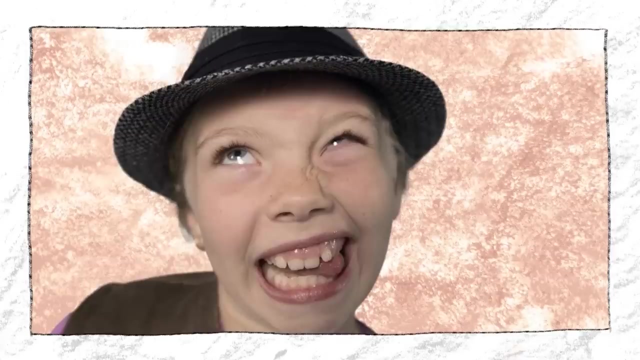 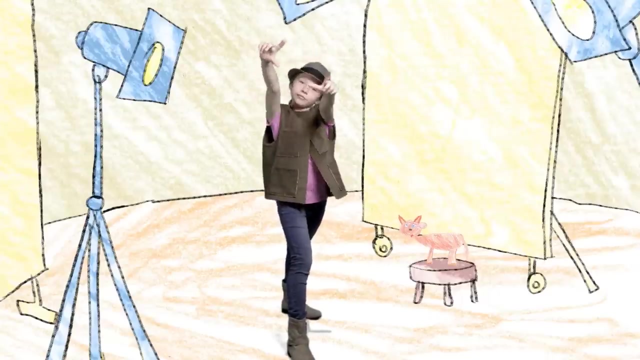 I would also take photos for the newspaper. My dad would jump up and down all excited whenever my photos are on the front page. Sometimes I would take pictures of me. Look at my selfie- Cheese Selfie, Smile. As a photographer, I would take photos of my own studio. 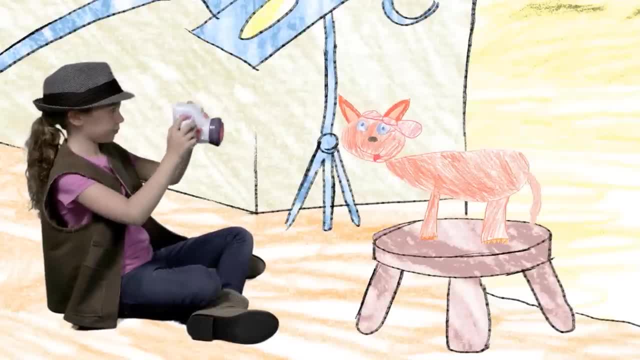 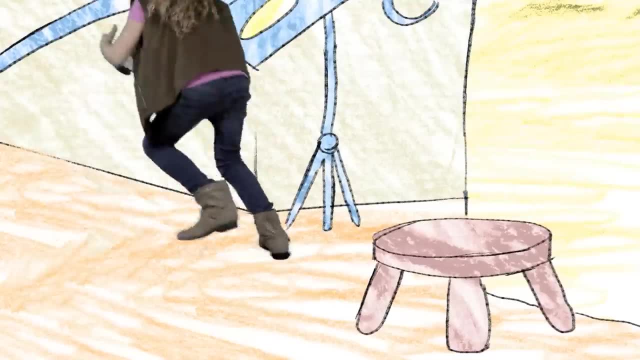 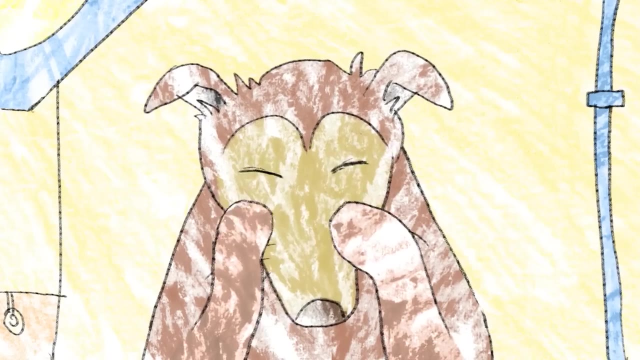 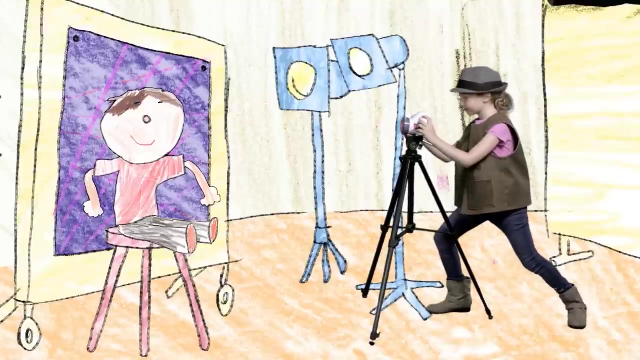 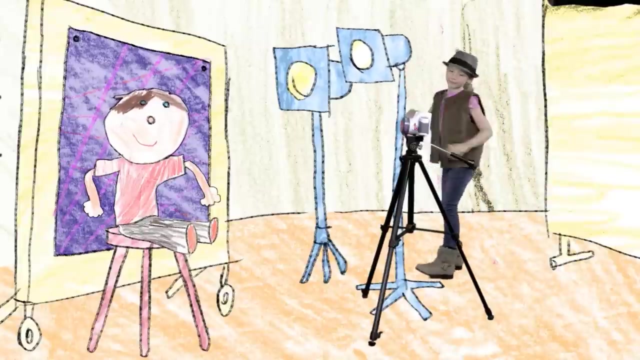 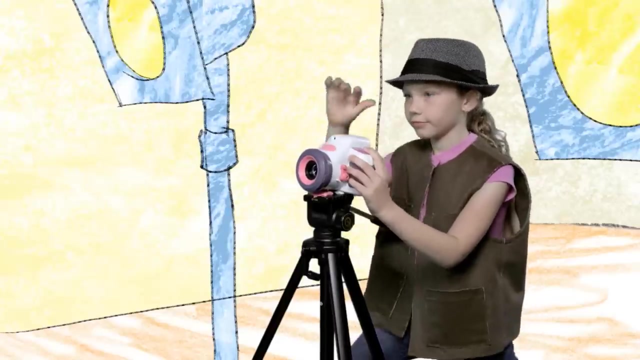 People would hire me to take photos of their pets- dogs and cats. Sometimes the animals would make funny faces Smile. I would also be hired to take school photos. I would adjust my lights to make everyone look their best. Cheese, Now look to your right. 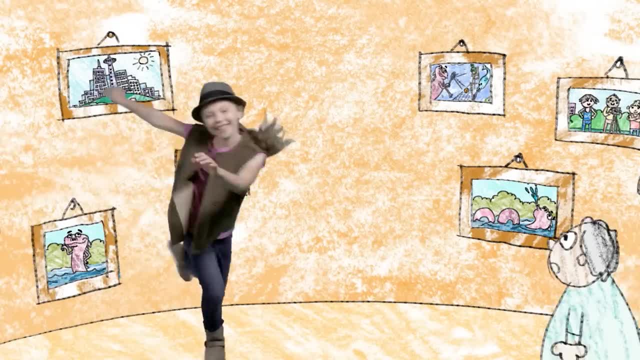 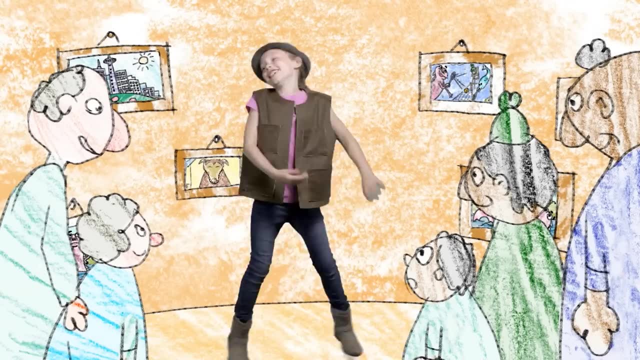 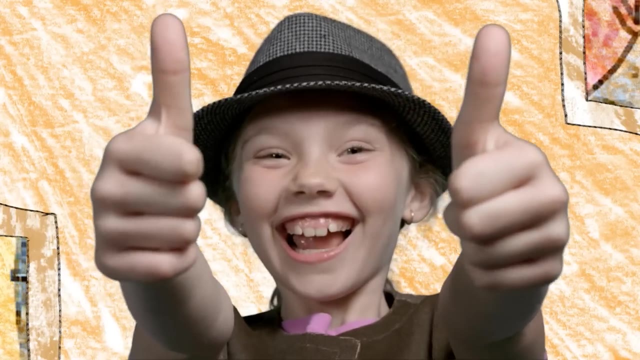 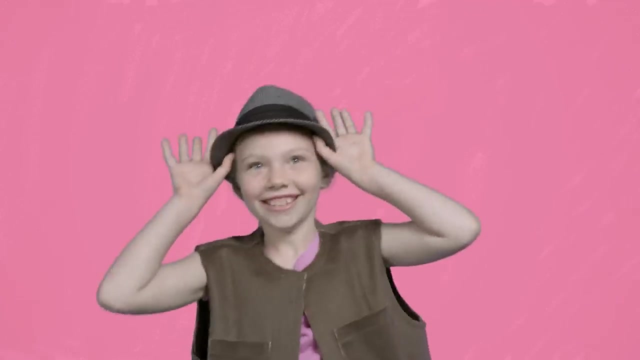 That's funny. I would select my favorite photos And display them in my own gallery. People would come from all over to see them. Being a photographer would be great Selfie. Can you imagine being anything you want to be? Can you imagine there's a world full of fantasy? 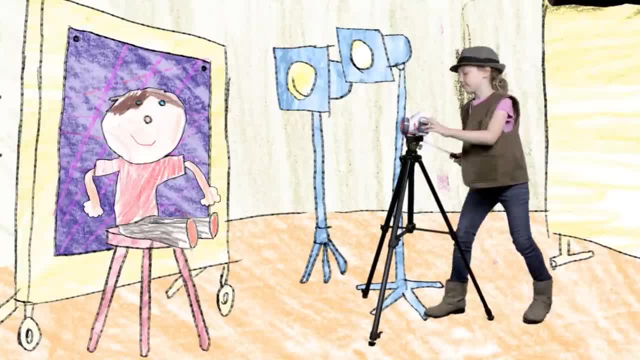 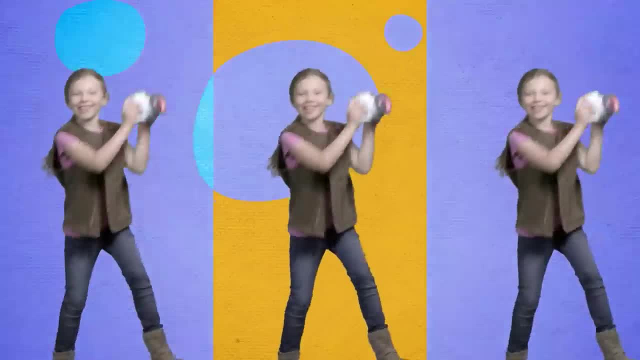 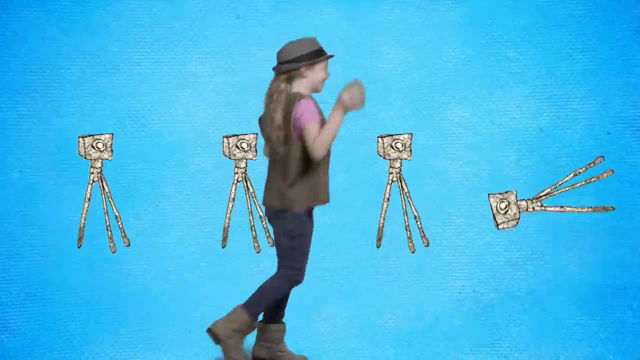